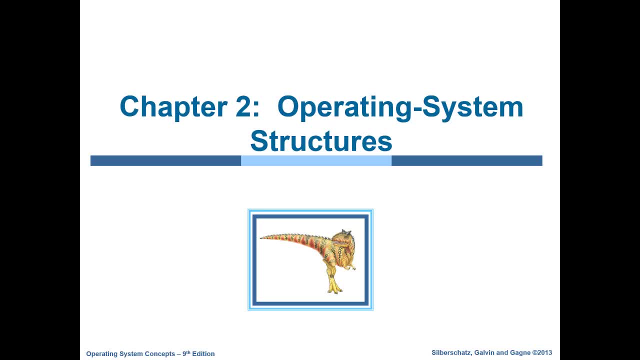 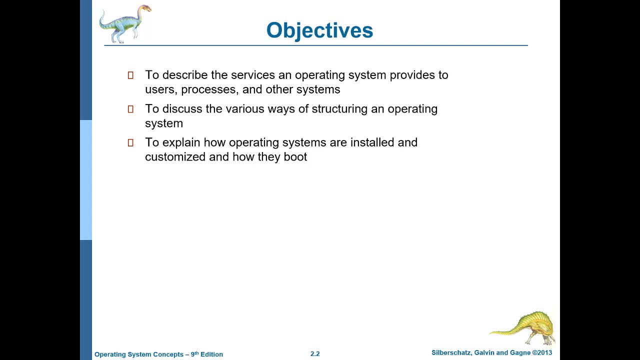 Okay, what is caching? And then in this chapter we are going to discuss the operating system structure in details. So first we described the operating system as a software which provides services. Operating system provides services to the users through processes and other systems, And then we will discuss the various ways to structure the operating system. 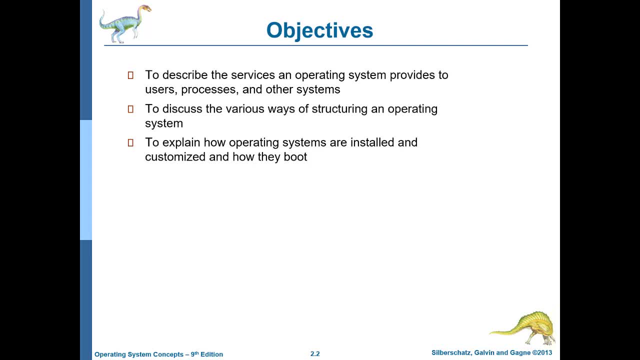 Okay, And then we will see different examples of operating systems and how they are different from one another. And finally, I hope you know how to install an operating system. In the course of introduction to operating system, you already learned how to install Unix or Linux system, Ubuntu system or Linux Mint. you have already installed, And then you should also know how to install Unix or Linux system. 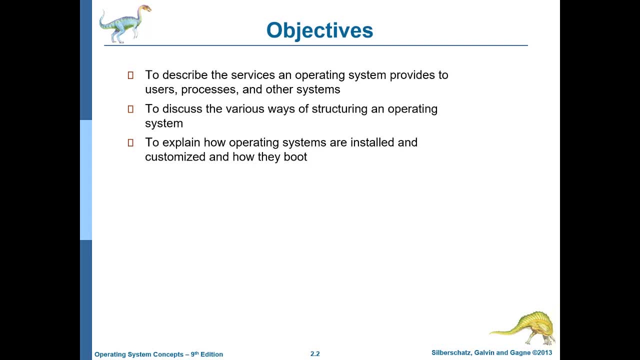 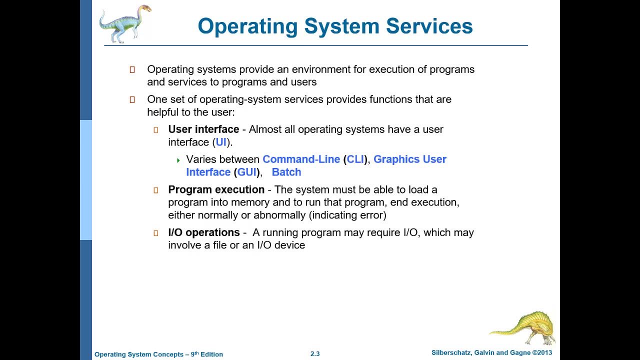 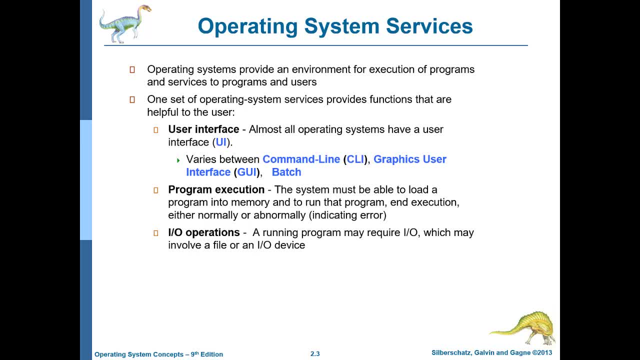 for execution of programs so is if there is no operating system, you cannot execute any program. that's one thing. the second thing is the operating system provides services to the programs and the users. so in general, operating system can have these functionalities, one which are related to the user interface. the other type of functionality is related 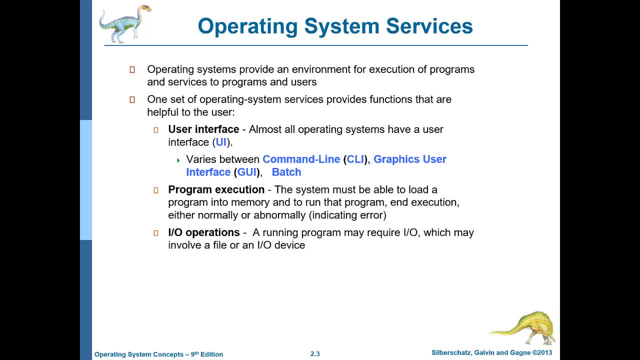 to the program execution. and third type is about the i operations and further we will see more things such as file system manipulation, communication, error detection, etc. we are going to discuss them one by one. so the first type of service provided by the operating system is that operating system. any operating system in general has a user interface and we can have different. 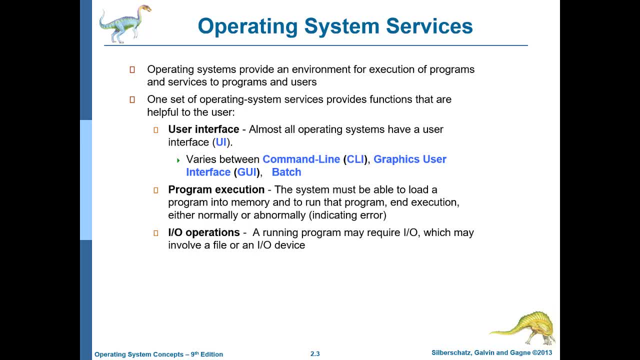 types of user interfaces. one type of user interface is the command line interface. can you give me an example of command line interface? do you know what is a command line interface? sorry, what unit instruction? no, no, no command line interface. if you remember from the course of introduction to operating system, then it's where actually you. 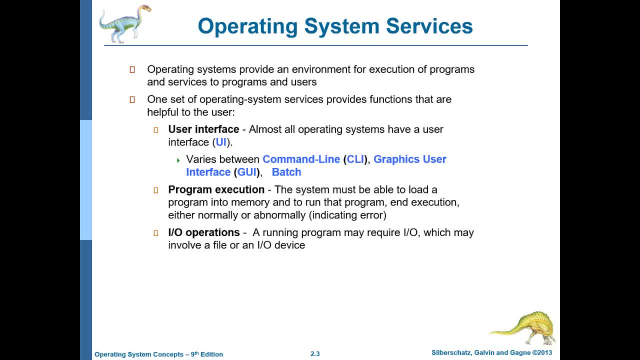 enter the command, for example, linux, terminal, or maybe here, in terms of windows, you have the command prompt. so a command prompt is actually where you execute instructions. so here in this window, i'm showing you the command prompt. you can have something like dir. okay, you cannot see it, okay. 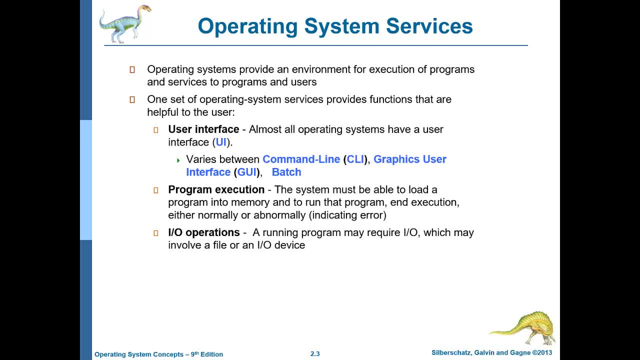 this way. let me show you the screen here. so this is an example of a command prompt. okay, so here i enter the command of dir. okay, so it shows me the contents of this directory. similarly you can do cd to move to some other directory and so on. so in command line interface you can enter commands. but 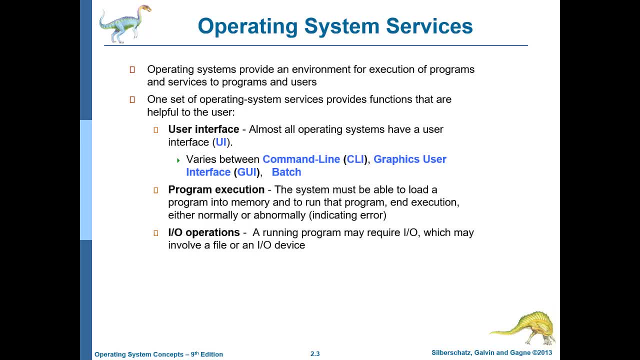 you don't use mouse, it does not have support for mouse, only the keyboard input. and when you enter a command, you press enter, the operating system executes the command. and when the command execution is finished, the operating system is waiting for your next command. in this example, now. 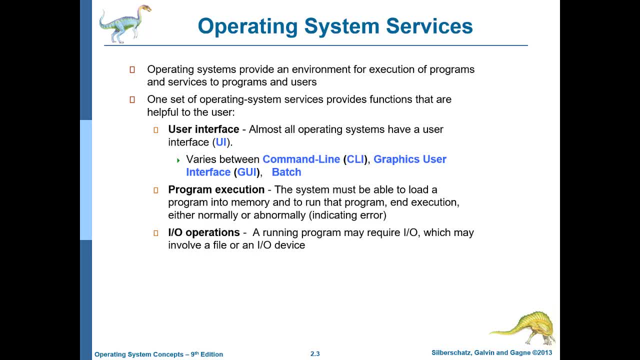 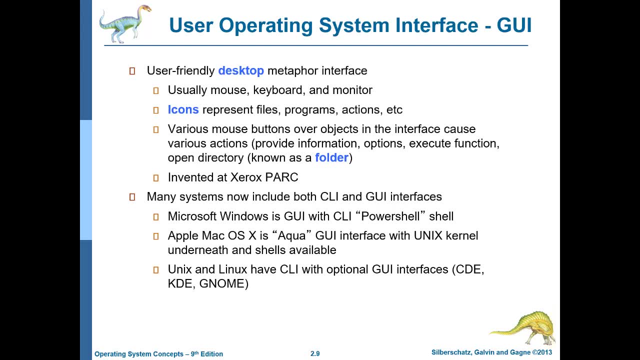 the operating system is waiting for my command. do you understand many of the systems. they include both command line interface and graphical user interface. okay, so for example, in microsoft windows, we have both the gui, which means the windows and menus and all those things, as well as the command line interface. okay, this is called powershell and i. 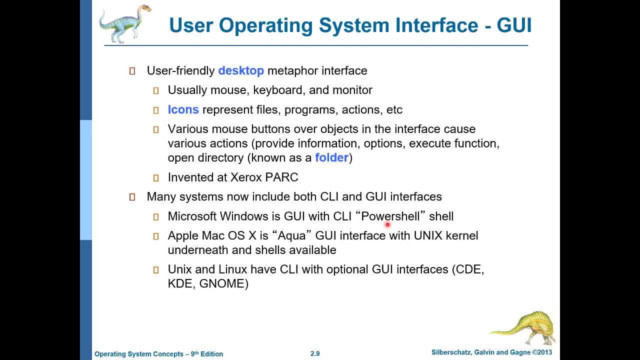 showed you before that if you run the cmd command it will open the command prompt, which is a command interface in the command window to user interface and useware to access the command interface. similarly, in mac os you also have the gi interface and the unix kernel and then both the unix and linux. 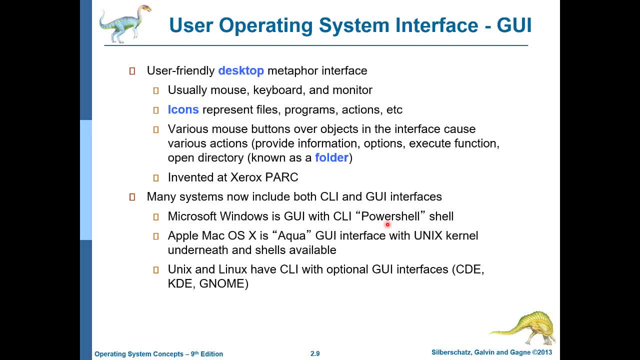 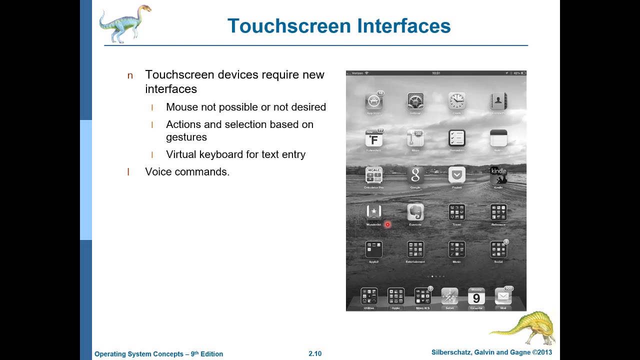 kernels. they have command line interface by default and you can also use the gui interface, and in linux and unix there are different gui interfaces available. you have the choice to use genome, KDE, CVE and there are many, many others Test screen interfaces. they are used in mobile devices and tablets and they do not support mouse. 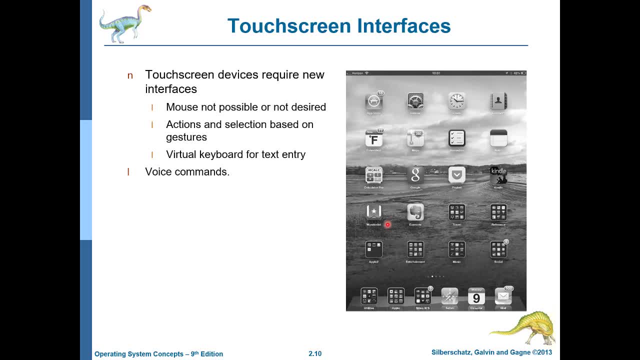 Instead you have to use fingers for various gestures. So you have one finger, two finger, three finger or up to four finger support for actually doing various types of actions: For opening applications, for changing screens, for doing other type of gestures inside the applications. 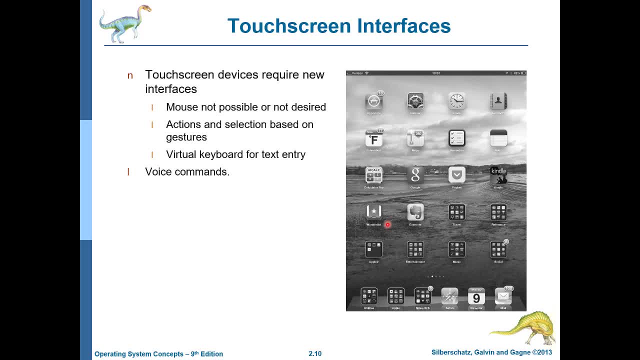 And finally, you also have voice commands, So you can talk to your device and it will carry out the command. Example: Google Assistant, and in iOS you have Siri. Finally, you can also have voice commands In Windows. There is something, an assistant, an application, which is called Cortana. 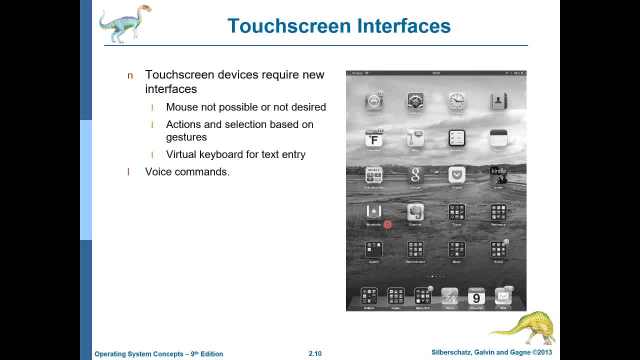 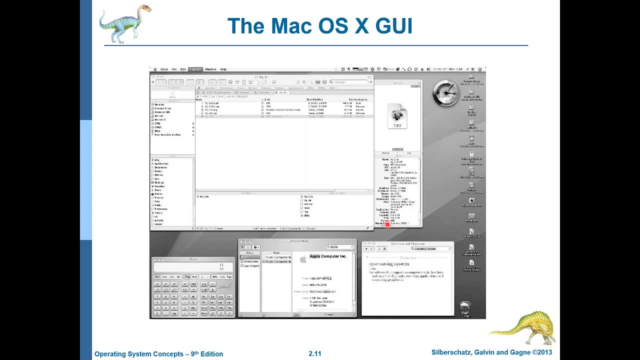 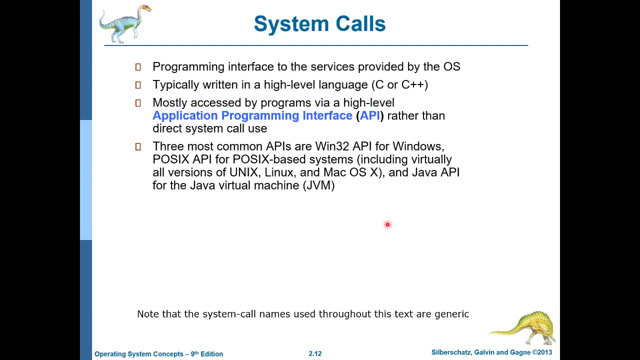 So the Cortana listens to you and it replies back or it acts on your commands. This is example of Mac OS X GUI. Now we come to the topic of system calls. What is a system call? We have discussed it a few times before. 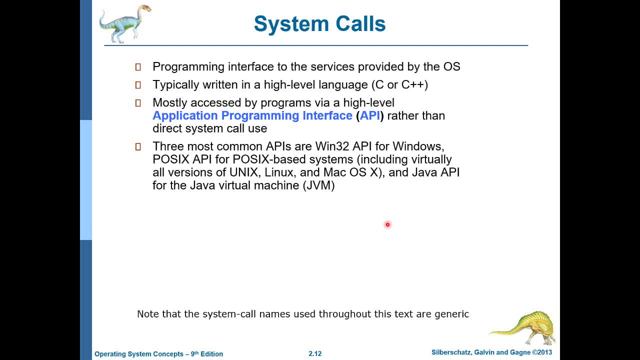 And here we are going to discuss it in detail. A system call is. A system call is actually the interface between your applications, or the user applications, and the operating system. Why? Because we discussed before, operating system provides different services And the programs which need those services. they use system calls to get access to those services. 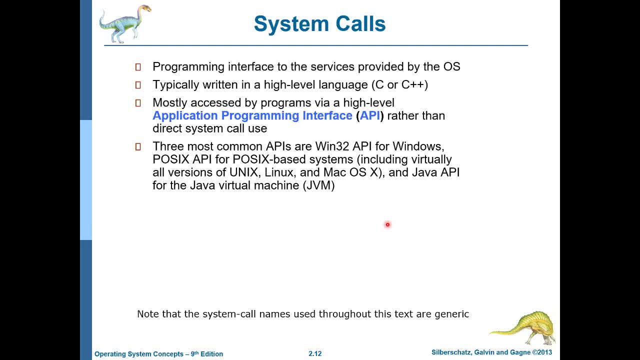 What type of services? We have seen services related to devices. We have seen services related to access of processor and RAM, Management of processes. What do you want to do with the process? Create a process, delete a process, terminate a process, abort a process? 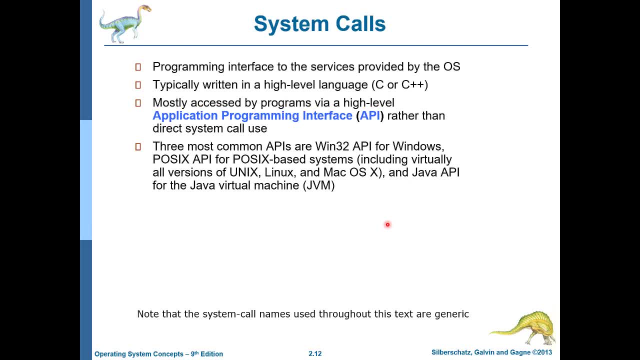 All of these, they require access to operating system. Do you hear me? So an operating system provides certain services And to access those services, the operating system also provides systems. Now, because you have different programming languages, for example C, C++, Java, Python, C, sharp, etc. 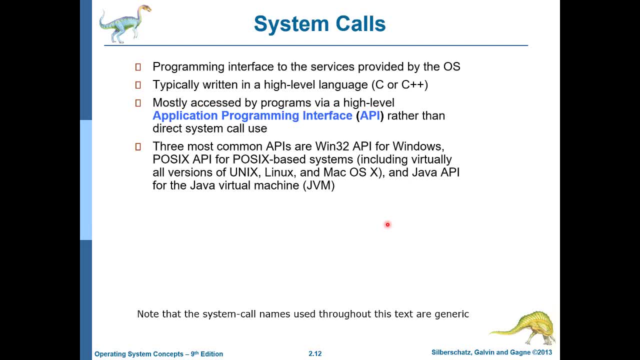 And operating system may be created in only one language, for example C. So how do they communicate? For this purpose, you have application programming interface. What is application programming interface or API? An API is actually a set of functions, a set of program code for a particular language. 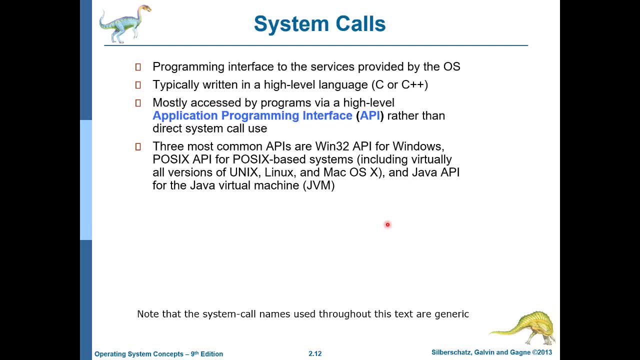 Which, in this case, will actually help you to access the system call interface. So if you are creating a program in the language of, in Java language, So Java has Java API And this API. you have different functions to actually call the system calls from your code. 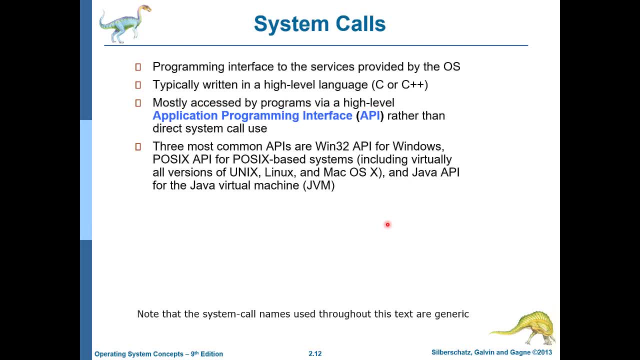 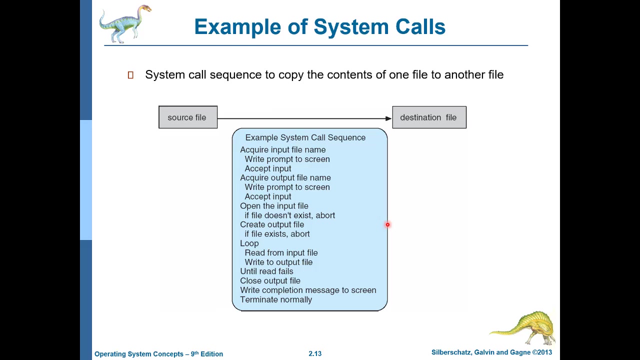 Similarly, you have Win32 API. if you are programming Windows- old Windows, New Windows- they have NET API. Then you have POSAX API And similarly, of course, Java virtual machine- you have Java API. This is an example of how do you copy content which are found in one file to another file. 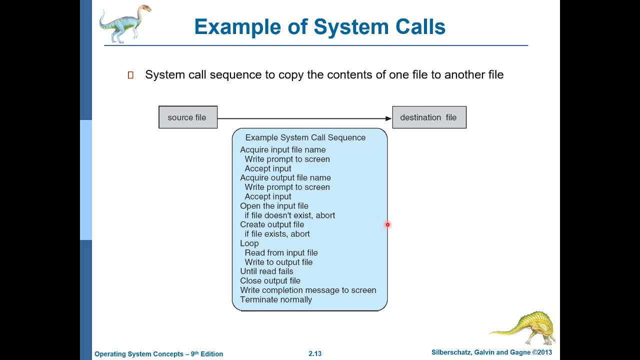 So you see here some steps of system calls which are executed by the operating system Or your program when it's called operating system And you can see that it starts from the input file link, Starting with the input file name, Then asking the user to write the input file name. 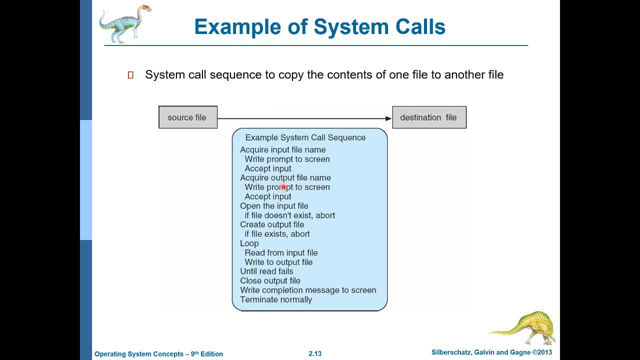 It accepts the input, Then it asks the user to write the output file name. It opens the input file, Then it reads the content from the input file And until the end it reads and write the output to the output file. After that it closes the output file. 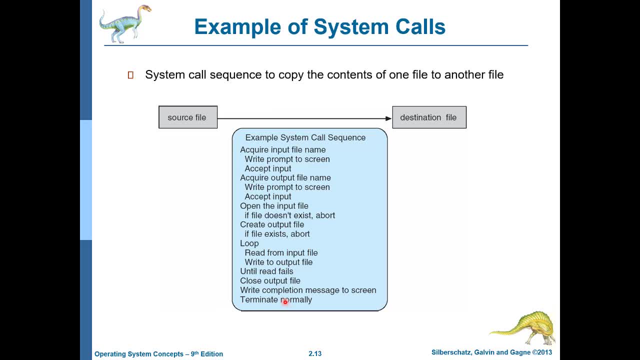 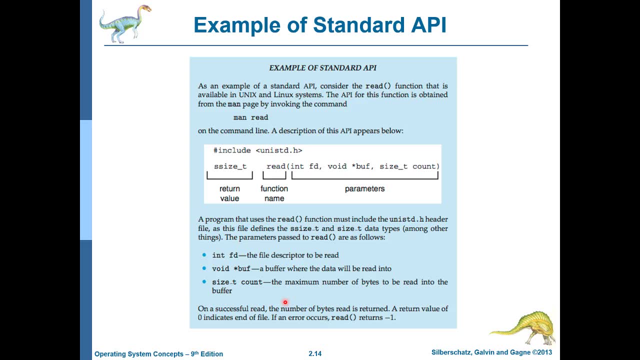 And then it terminates. Every step is actually a system call. This is the example of standard API: the read function. It has file descriptor- The first argument. The second argument is the buffer And then the number of bytes you want to read. 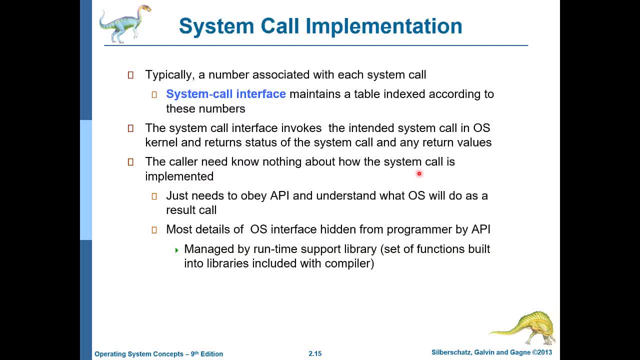 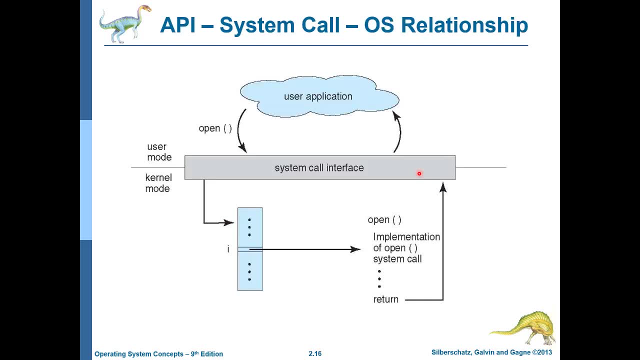 We have, I think, already discussed this, So I will just move to the next thing, which is: how do you implement system call? So, for that purpose actually, you have a table, System call table, And in this table you have a number, some digit or an integer number actually. 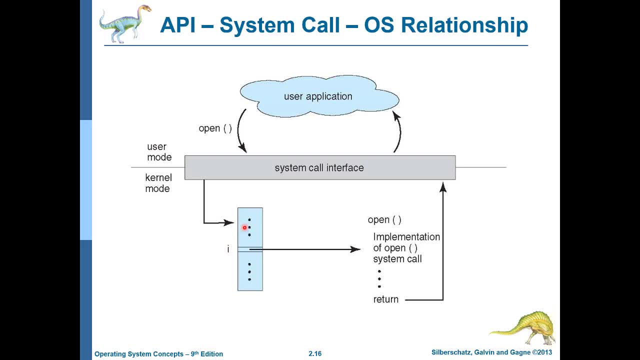 And that number corresponds to a system call. So the operating system knows which number corresponds to which system call And the application. when it calls some function, the operating system finds the math and opens this system call, runs it And the result is returned back to the user application. 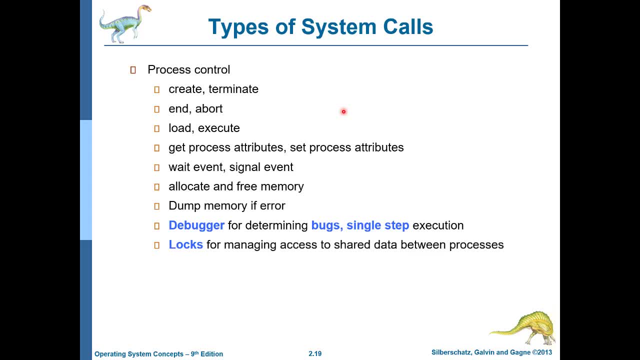 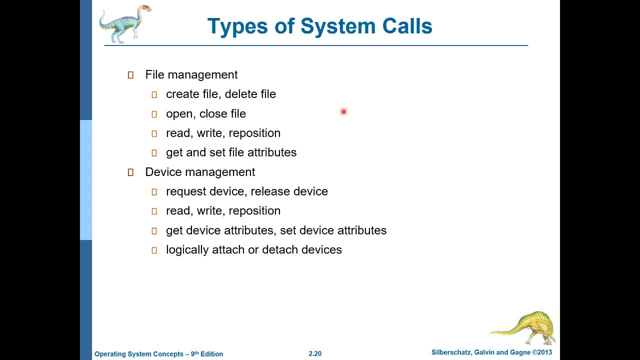 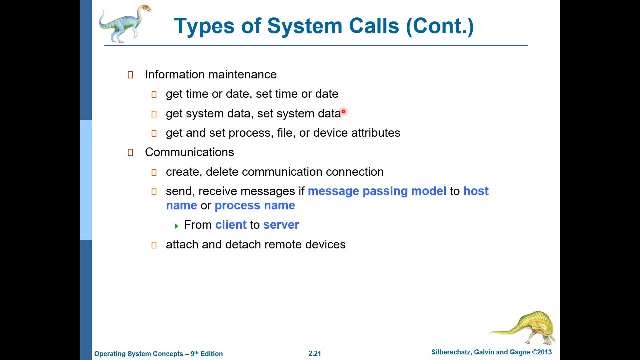 Now there are different types of system calls: System calls for process control- You can see there is a big list of system calls for process control. Then there are system calls for file management and device management- We have discussed that before- And there are system calls for information maintenance. 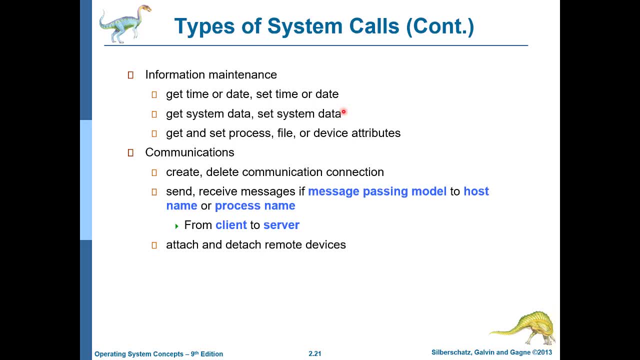 For example, to get time or date, to set time of date of the system. Similarly, other system data System information, user information, region information, language information. There are system calls for these things. You have communication related system calls. 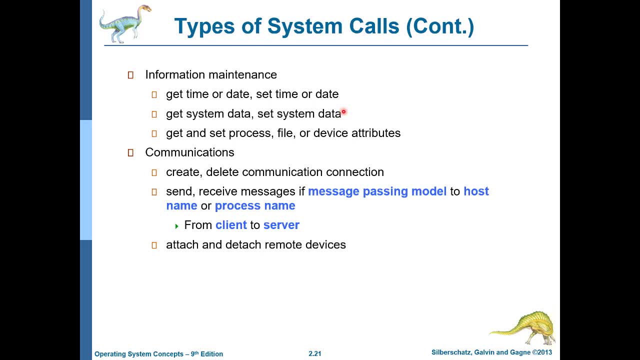 When different processes they communicate with each other, And how to attach and detach remote devices. Now, system calls. One final thing about system calls, About protection related system calls. So if you want to change some attributes of different resources To make it readable, writable or executable, 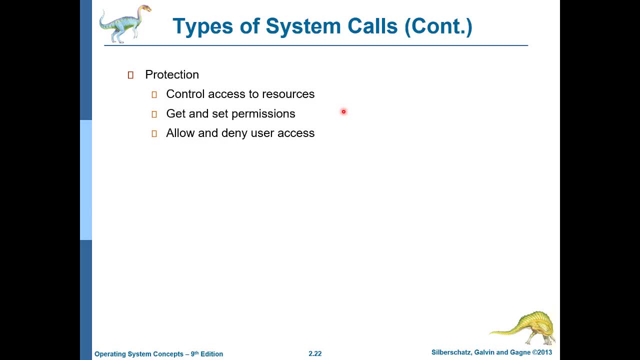 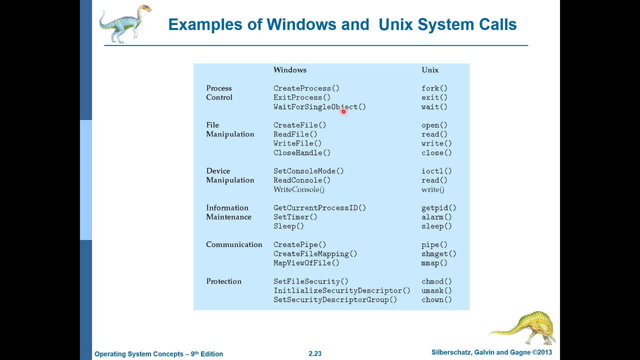 Or to make, get and set permissions, Or to allow or deny users to access something. These are different system calls. This example is actually a comparison of system calls that you will use in Windows and Unix, And their objective is the same. So these are actual Windows 32 API system calls. 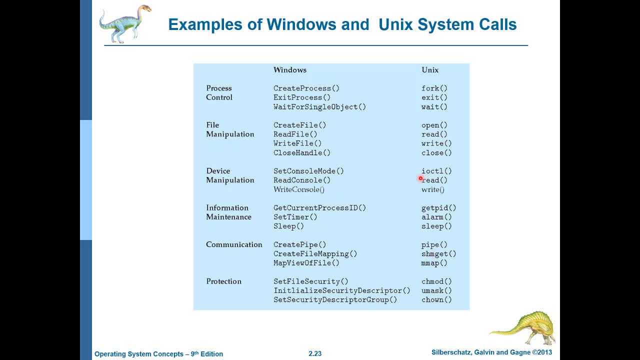 And these are Unix project system calls Two different application programming interfaces, Or system call libraries For each of these operating systems. So for creating a process, you have create process, And for deleting a process, you have exit process, And so on. 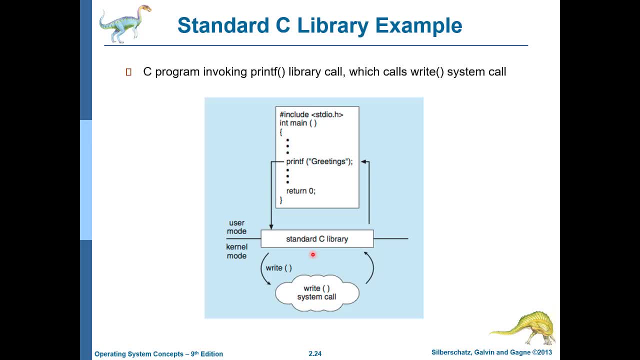 Now, in this example, what you see Is that even a simple command like printf That you are going to use in your program Printf, and then some message: This actually uses a system call. So printf is a standard C library function And it is implemented in terms of write system call. 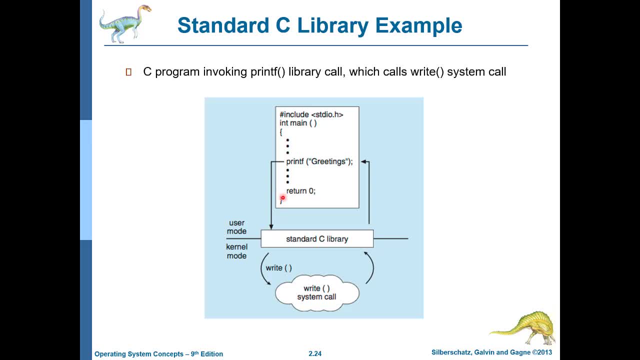 So when you ask printf command, It will execute the write command in the system call of the Windows or Linux operating system. The write system call will execute it, It will write something onto the screen And then it will return the control back to your program. 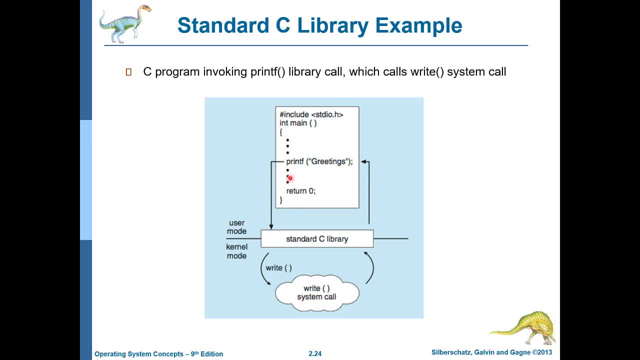 The important thing here is to note That when you are executing a standard C library command, It is in user mode, But when you want to execute, Or the operating system wants to execute, a system call, It will change to kernel mode When the system call execution is finished. 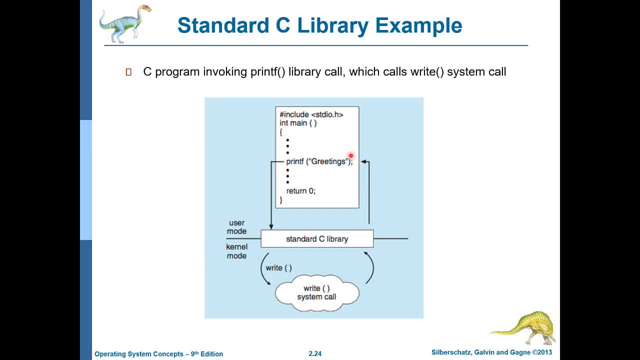 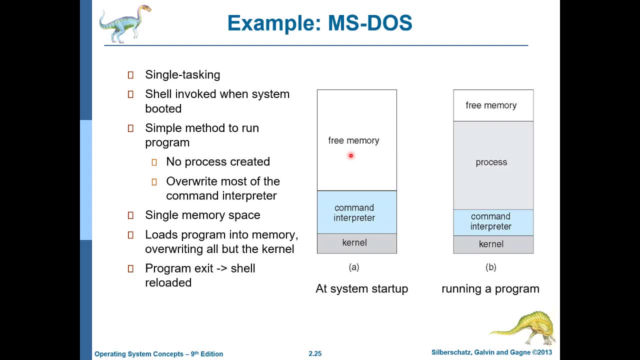 The control will return back to the program in the user mode. Now we are going to study some example operating systems. The first one is Microsoft DOS, And then we will study UNIX, Android and iOS as well. Now what you see here: Microsoft DOS. 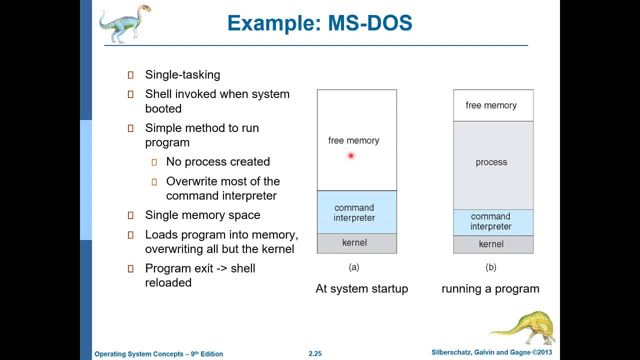 It was there in early 80s until 90s. This DOS stands for Disk Operating System. This is a single tasking operating system. What is single tasking? Can anyone tell me? Single tasking operating system: Only one program can be executed at one time. 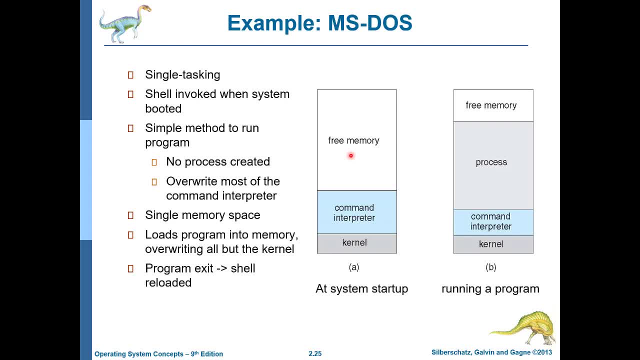 So when you load a program You cannot execute any other program. You have to finish the program And then the control will return back to the operating system. Then you will execute another command To run another program, and so on. So this is single tasking. 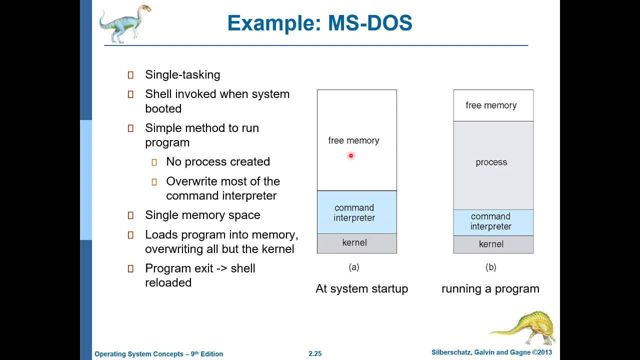 And even now, if you run MS-DOS, For example, let me explain. If you buy these days, If you buy a laptop from extra, for example, So they will not give you Windows For most of the laptops Because the Windows license is very expensive. 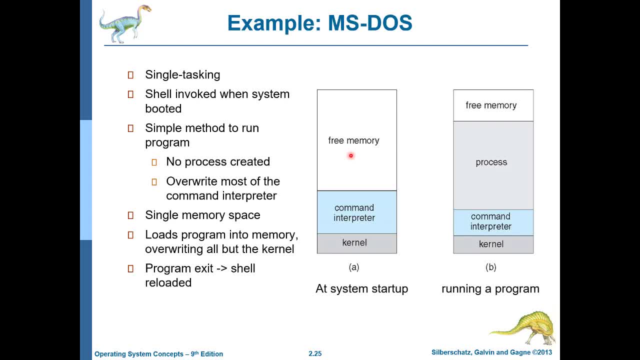 So they will give you MS-DOS installed, Or you have to buy Windows And then they will install Windows for you. So MS-DOS is there. You can test that, Or even you can download MS-DOS online And test in your operating system. 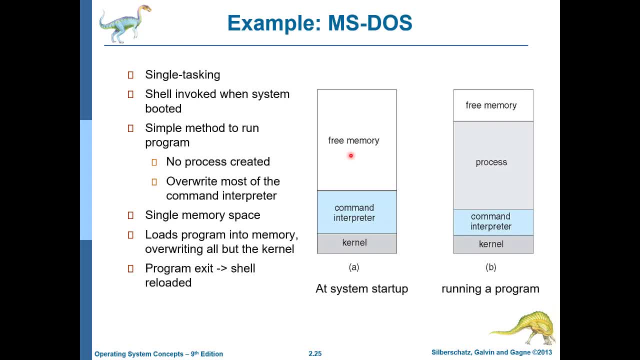 But since MS-DOS is already there As command shell- Not completely, But commands of the MS-DOS are there in the command shell So you can execute the command. So the shell is invoked When the system is booted And this shell needs what? 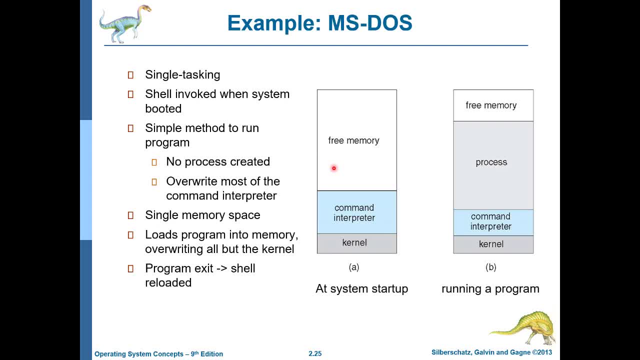 We will enter the command. So actually very simple thing is that When you run a process It is created in part of the commands prompt And when the process is executed, The command interpreter or the command prompt comes again And there is stream memory to run more programs. 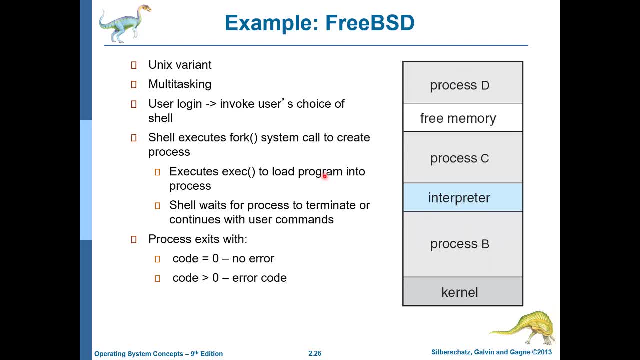 FreeBSD is an example of UNIX. This is a type of UNIX. This is a multitasking system And you can see there are many processes. So when you started Maybe you had process A And process A, execution finished. So you run process B, process C, process D. 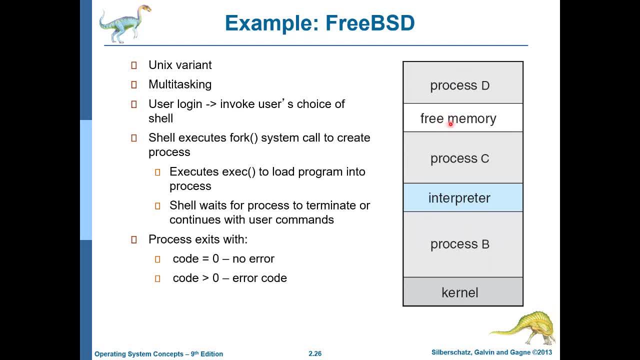 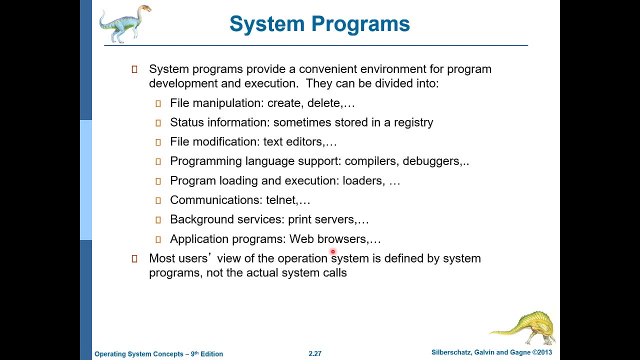 And still there is some free memory. You can have more processes run inside this free memory And also the interpreter is always available alongside the kernel in the memory. Now we study about system programs. What are system programs? These are different programs Which are useful for carrying out different activities. 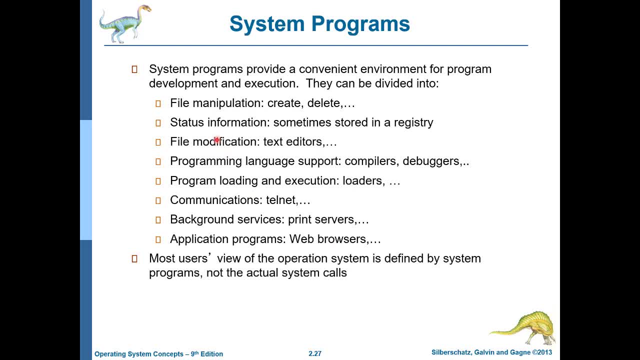 Such as creating or deleting files, Status information And all those other information. Example is: in Windows you have the program which is called file explorer. Similarly, you have program like notepad or wordpad And you have programs For printing. You have programs for connecting with http or telnet or fcp, etc. 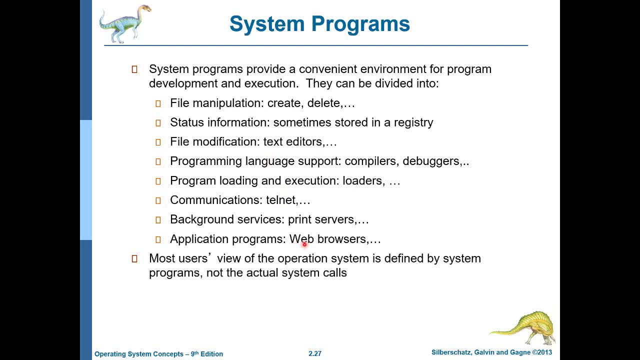 These are different programs. The important thing here is that the users- They know the application programs or the system programs, But they don't know the system calls For them. the application programs are the important thing, Not the system calls. Okay, So system programs. 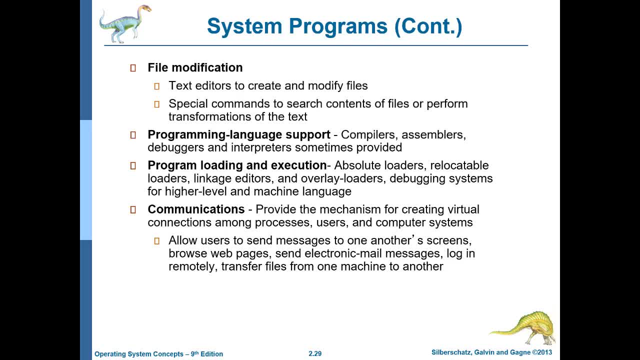 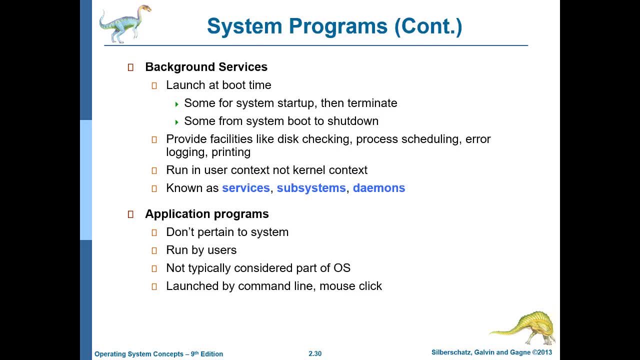 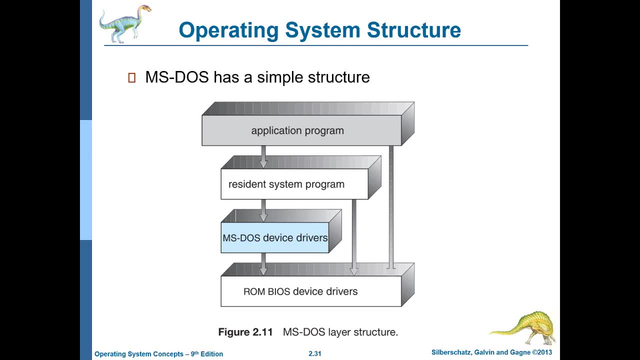 This is an example. This is a list of examples of system programs. You should go through them. Okay, We have to do it very quickly Because we are running short of time. Okay, And operating system structure of MS-DOS. This session will discuss some structures of some operating systems. 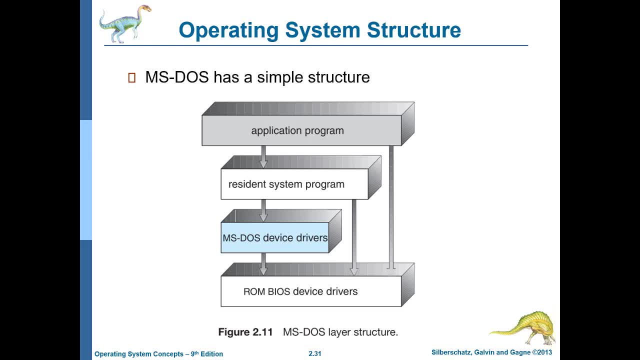 For example in MS-DOS. what do you see here? That you have these different layers. Okay, So at the bottom, Near the hardware, You have device drivers Which are for ROM, BIOS device drivers, Then you have MS-DOS device drivers. 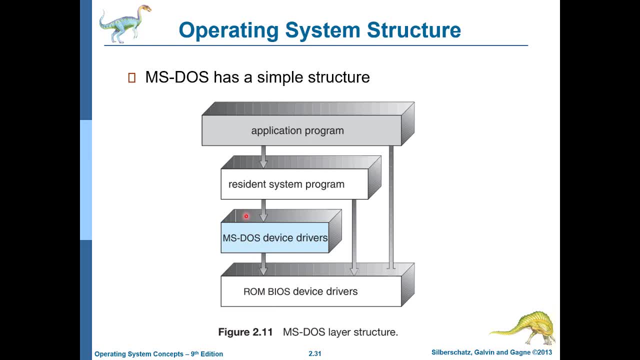 Which will communicate with the ROM device drivers. You have the resident system program, Which is part of the operating system. You can call it as the kernel Which is always there in the operating system In the RAM. Okay, This is called resident program. 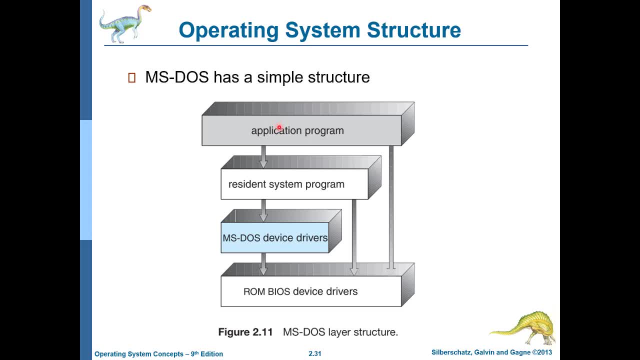 Which will be there Always. And finally, You have application programs. These programs are only in the RAM When you execute them. When they finish execution, They are terminated. These programs are: This program, Which is a single program Which is removed from the RAM. 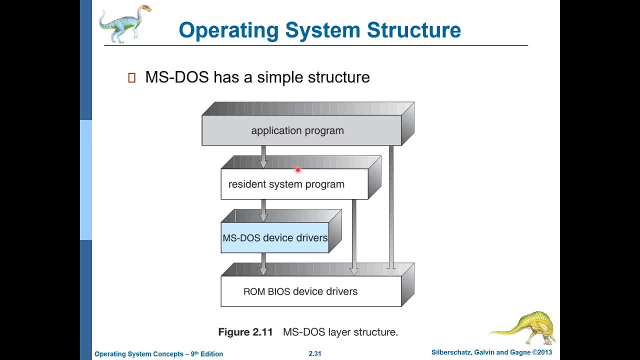 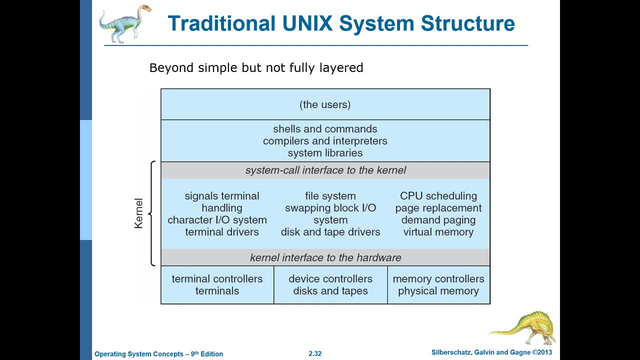 And another program may be loaded. So this is a very simple structure. The second example is that of UNIX system structure, And in UNIX system structure You have again different layers, Okay, But the important thing is That here the kernel is advanced. 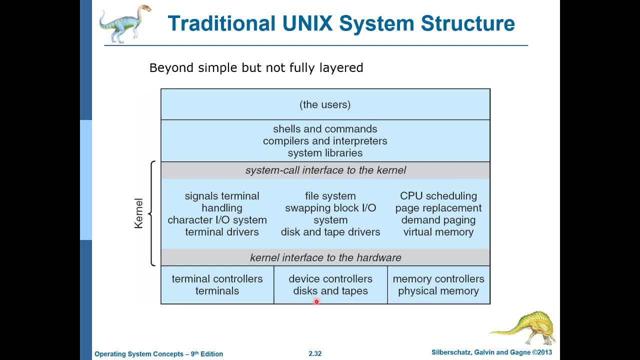 So you have an interface between the hardware And the operating system And another interface between the applications- Okay, System applications or user applications- And the operating system. So there are two interfaces: One to the hardware And one to the operating system. 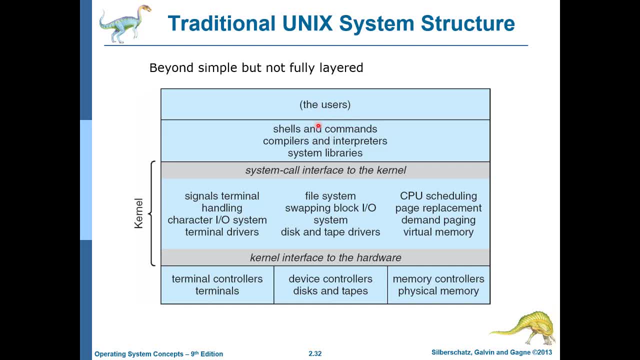 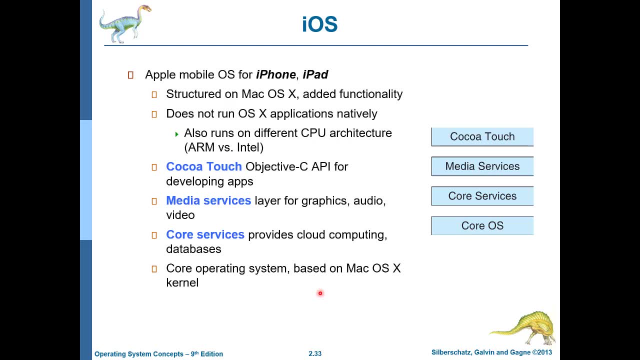 And finally, the user. They use these applications To do the tasks of the hardware, Use hardware To carry out their tasks. IOS structure At its base. It has core operating system. Okay, It is based on Mac OS structure, On core operating system. 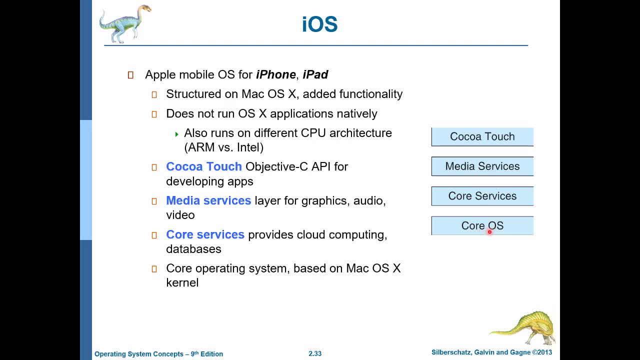 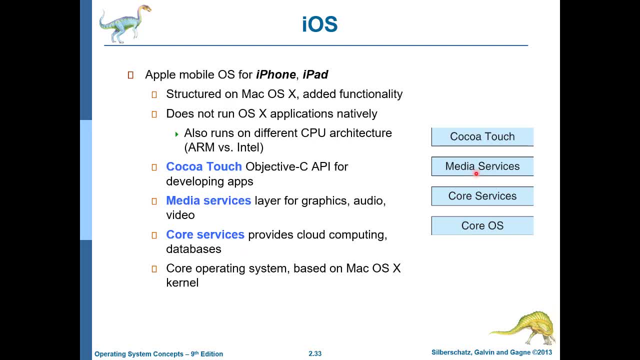 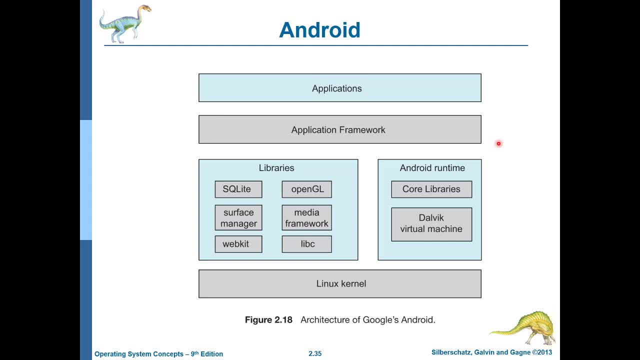 iOS. But important thing Is that It is a modified Linux Kernel, Okay, And it has 2 important aspects on top of Kernel. One is the set of libraries And the other one is the Framework. Okay, Which, sorry?